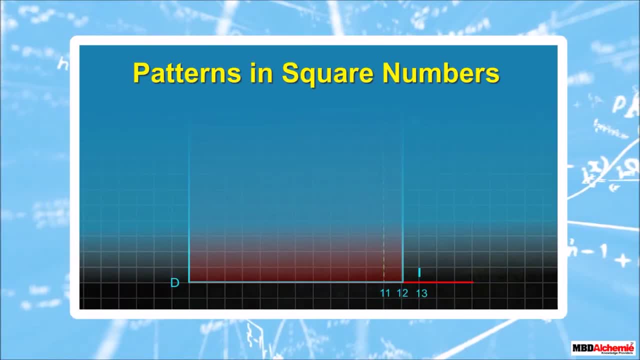 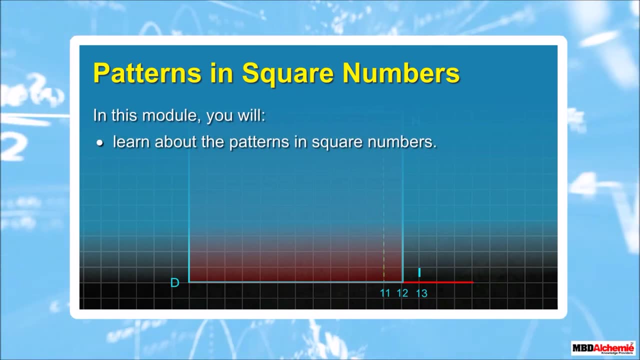 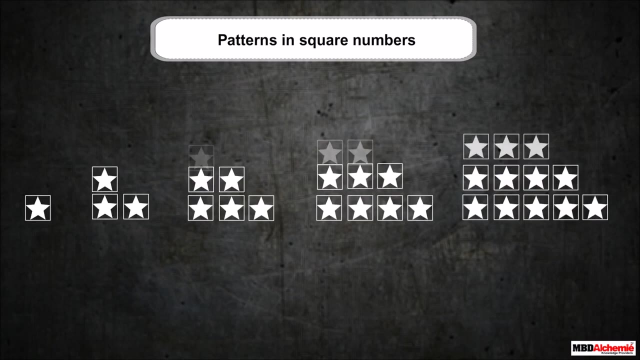 Patterns in Square Numbers. In this module you will Learn about the patterns in square numbers. Let us learn some interesting patterns in square numbers. Do you know the pattern shown above? These are the triangular numbers whose dot patterns can be arranged as triangle. 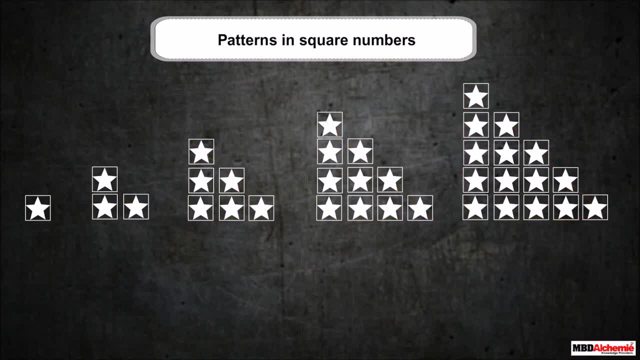 Now we combine two consecutive triangular numbers, like we add 1 star to 3 stars and get 4 stars. Similarly, we add 3 stars to 6 stars and get 9 stars. Then we add 6 stars to next consecutive stars. 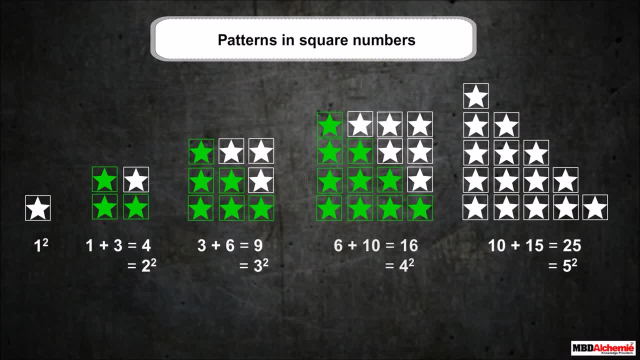 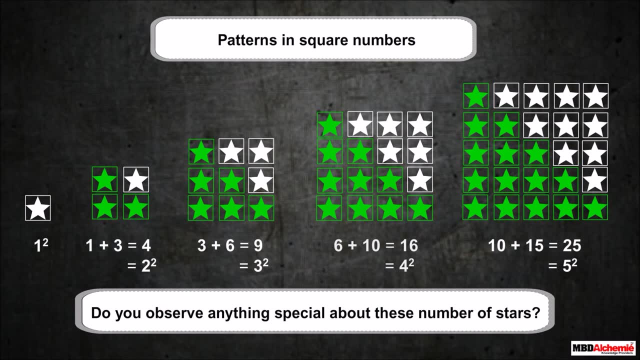 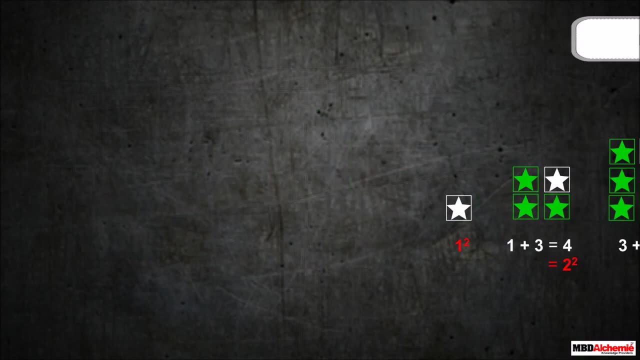 that is, 10 stars. We get 16 stars. Do you observe? Do you observe anything special about these number of stars? We get a square number of stars. Let's see the multiplication grid up to 100.. Now we shape the square numbers like: 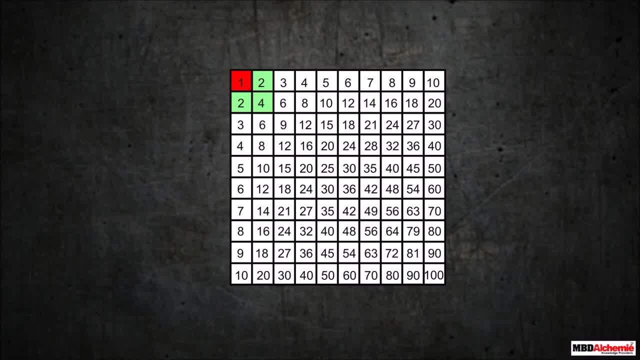 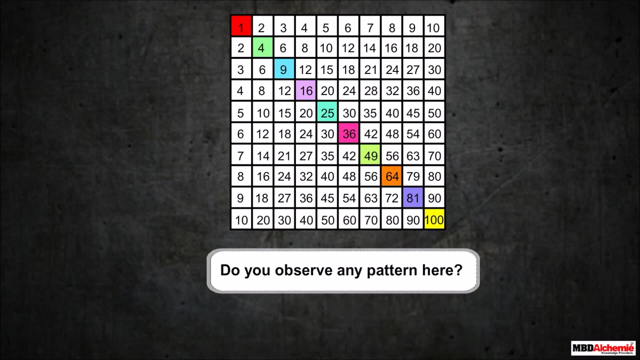 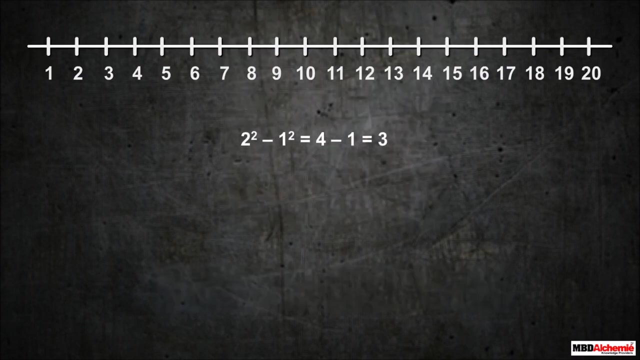 1, 4, 9, 16, 25, 36, 49, 64, 81, 100. Now what do you observe? Do you observe any pattern here? All the diagonal numbers are square numbers. Find the difference of square of 1 and the square of 2, that is 3.. 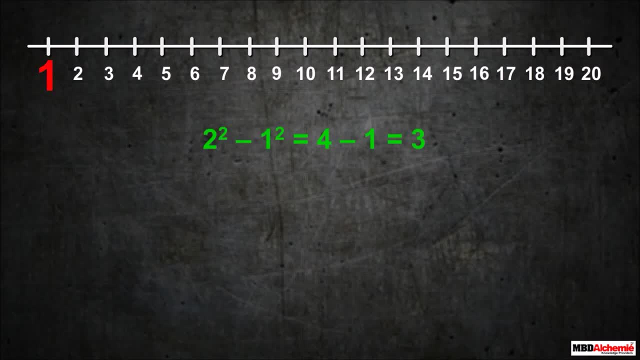 Now count the non-square numbers between square of 1 and square of 2.. There are two non-square numbers. Find the difference of square of 2 and the square of 3.. That is 5.. Now count the non-square numbers between square of 2 and square of 3.. 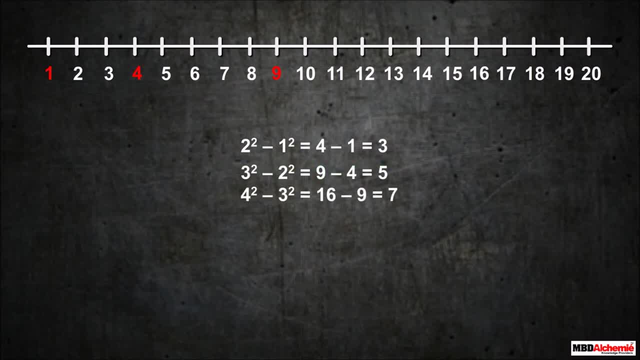 There are four non-square numbers. Again find the difference of square of 3 and the square of 4.. That is 7.. Now count the non-square numbers between square of 3 and square of 4.. There are six non-square numbers. 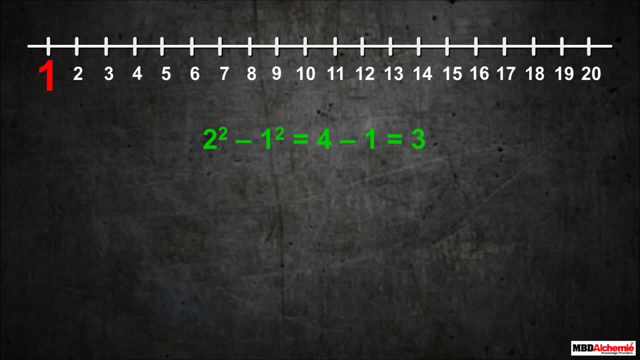 You can comment below for happening predictions. We hope you found the instructions helpful. Now count the non-square numbers between square of 1 and square of 2.. There are two non-square numbers. Find the difference of square of 2 and the square of 3.. 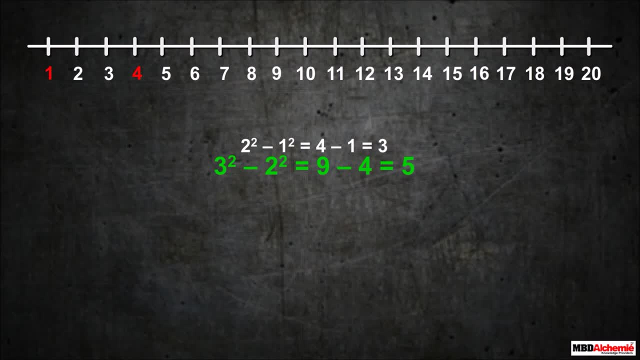 That is 5.. Now count the non-square numbers between square of 2 and square of 3.. There are four non-square numbers. Again, find the difference of square of 3 and the square of 4.. That is 7.. 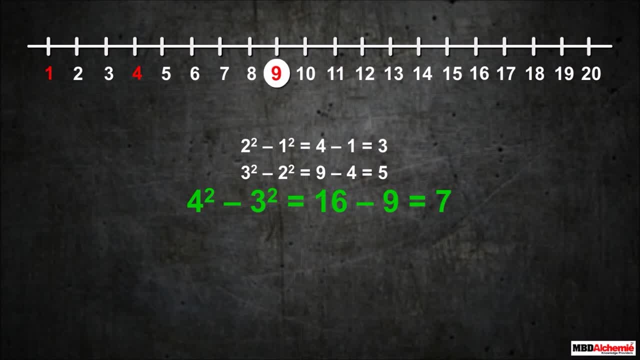 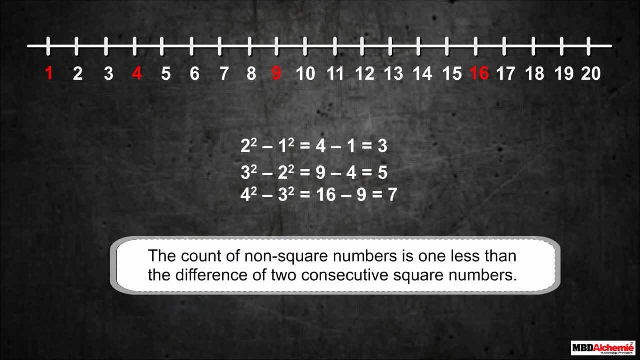 Now count the non-square numbers between square of 3 and square of 4.. There are 6 non-square numbers. Do you see any pattern? Observe the difference of the square of any two consecutive numbers and the count of non-square numbers between them. 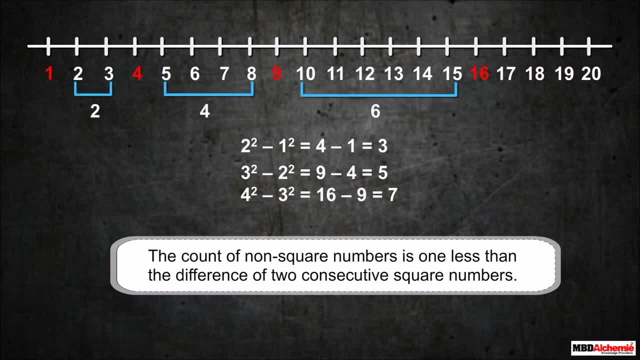 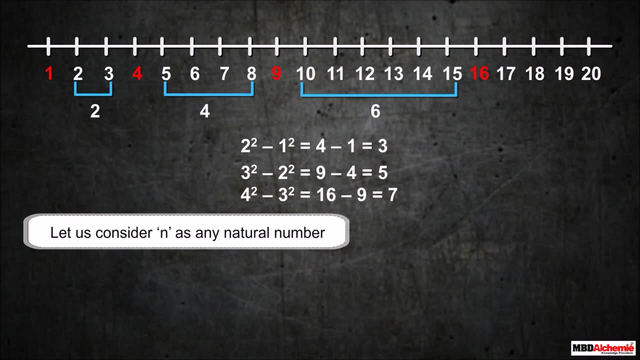 We find the count of non-square numbers is 1 less than the difference. Thus we can generalize this pattern in finding non-square numbers between two consecutive square numbers. Let us consider n as any natural number. Therefore its consecutive number is n plus 1.. 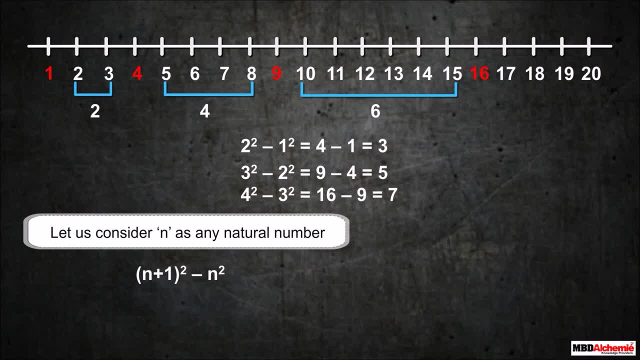 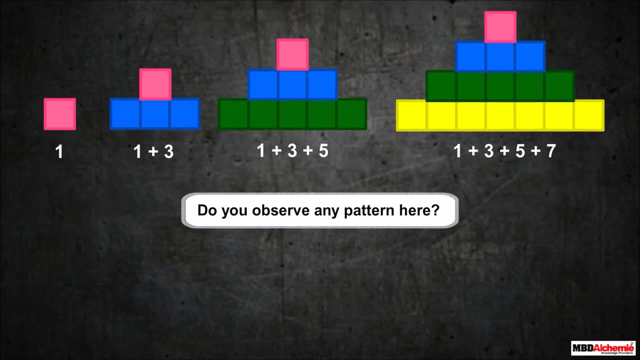 Then we write their difference in the square as n plus 1 whole square minus n square. This is equal to 2n plus 1.. Here are some stair-step patterns. Here are some stair-step patterns. Do you observe any pattern here? 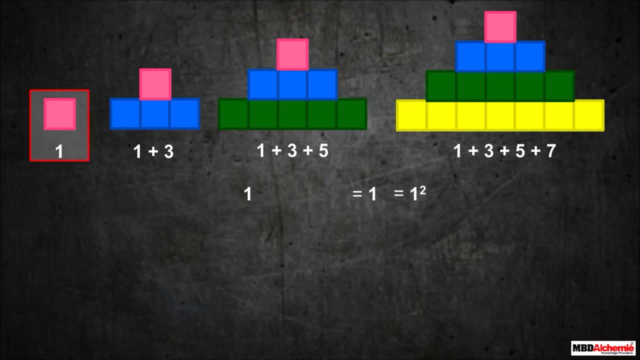 Now consider the following: The square of 1 is 1.. Then the sum of 1 and 3 is 4,, which is written as 2 square. The sum of 1 and 3 and 5 is 9,, which is written as 3 square. 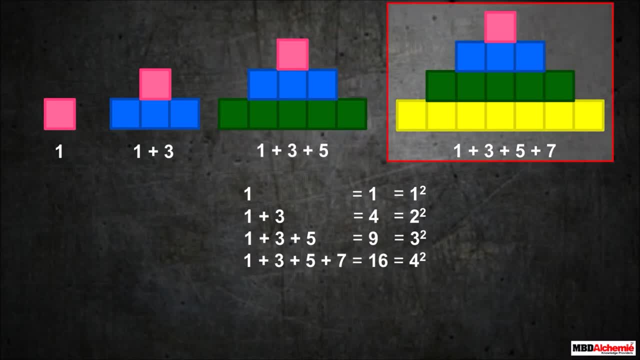 Similarly, the sum of 1 and 3 and 5 and 7 is 16,, which is written as 3 square. The sum of 1 and 3 and 5 is 7,, which is written as 2 square. 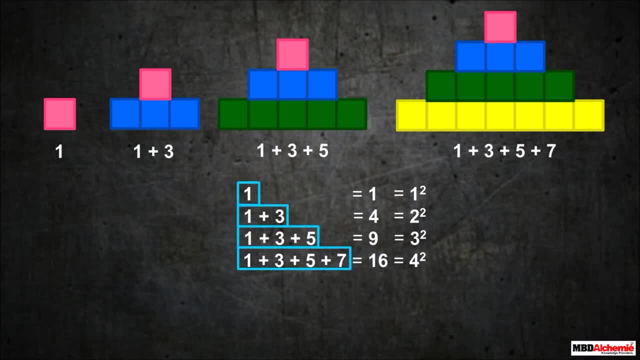 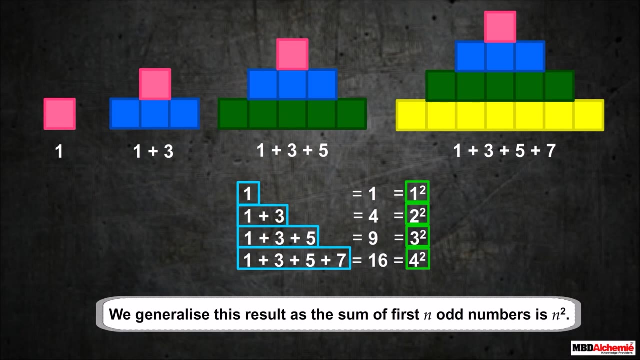 Here we observe on the left-hand side equality. There is the sum of odd numbers. On the right hand we get the square number. We generalize this result as the sum of first n-odd numbers is n squared. Let us consider the following. 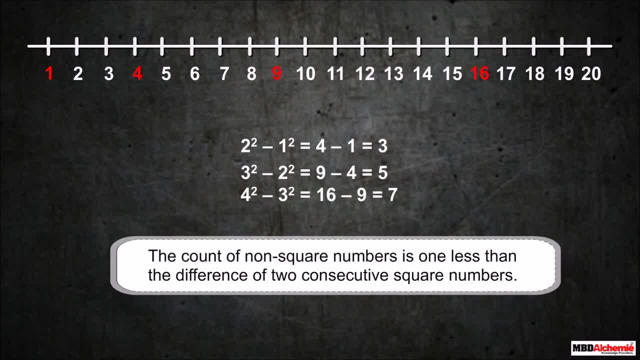 Do you see any pattern? Observe the difference of the square of any two consecutive numbers and the count of non-square numbers between them. We find the count of non-square numbers is one less than the difference. We can generalize this pattern in finding non-square numbers. 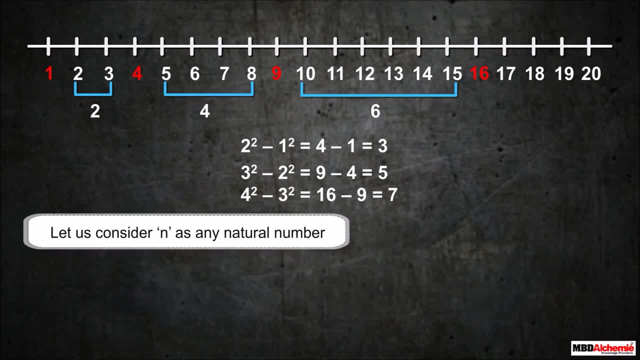 between two consecutive numbers. Let us consider n as any natural number. Therefore its consecutive number is n plus 1.. Then we write their difference in the square as n plus 1 whole square minus n square. This is equal to 2n plus 1.. 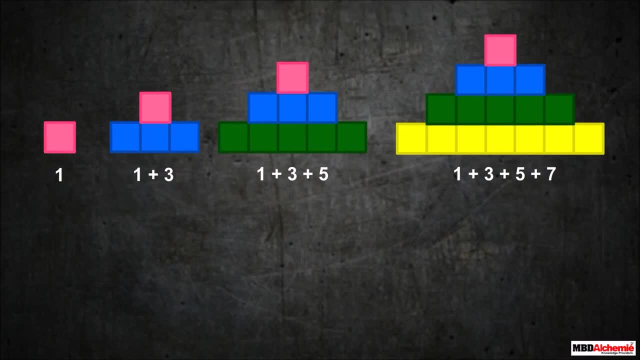 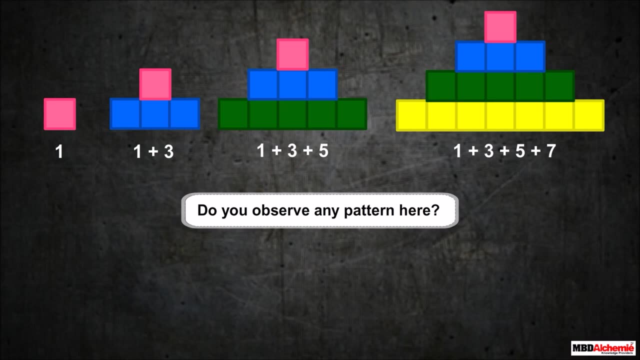 Here are some stair-step patterns. Do you observe any pattern here? Now consider the following: The square of 1 is 1.. Then the sum of 1 and 3 is 4,, which is written as 2 square. The sum of 1 and 3 and 5 is 9,. 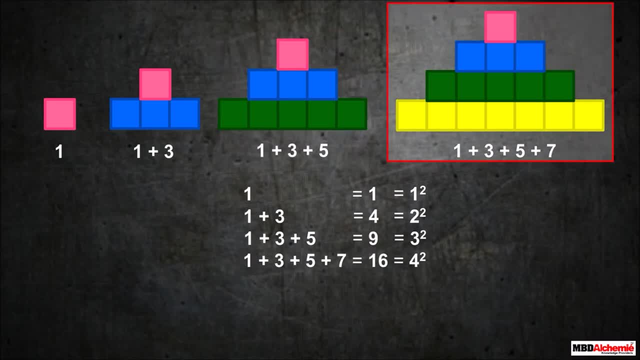 which is written as 3 square. Similarly, the sum of 1 and 3 and 5 and 7 is 16, which is written as the square of 4.. Here we observe on the left-hand side of the equality. 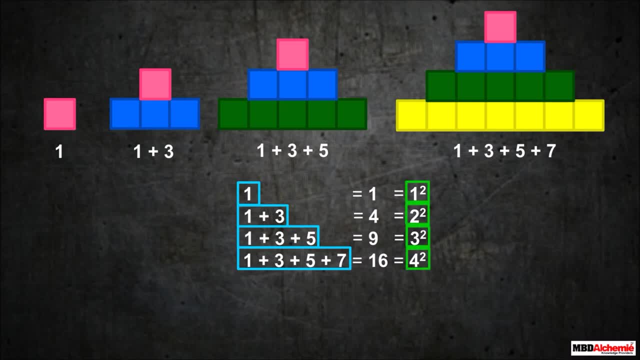 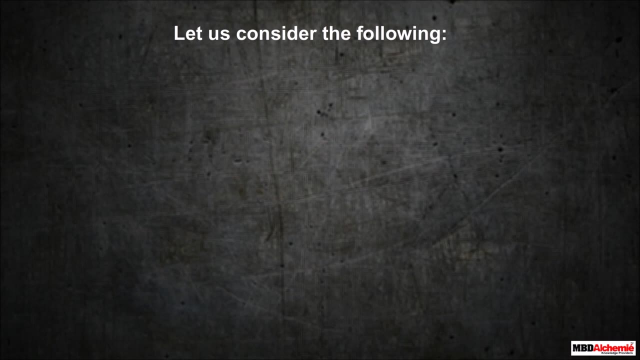 there is a sum of odd numbers and on the right-hand we get the square numbers. We generalize this result as the sum of first n odd numbers is n square. Let us consider the following: We can express the square of odd numbers as the sum of two consecutive numbers. 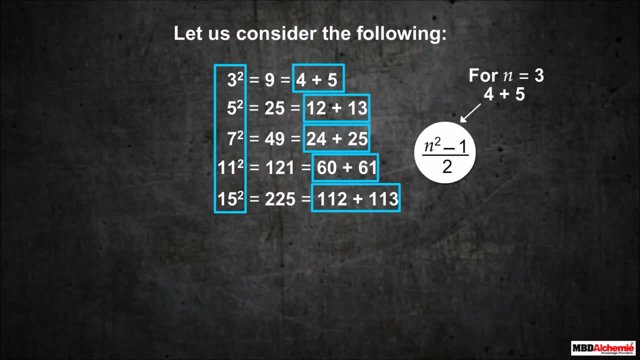 We find the consecutive numbers. We can express the square of odd numbers by subtracting 1 and dividing by 2.. And we find another number by adding 1 and dividing by 2.. Now let's take the square of an even number. 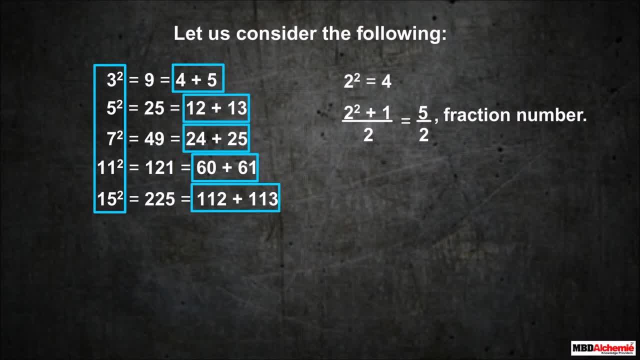 We find a fraction number instead of a natural number. So we say that this pattern is made only for square of odd numbers. We can express the square of odd numbers as the sum of odd numbers. So we can express the square of odd numbers as the sum of two consecutive numbers. 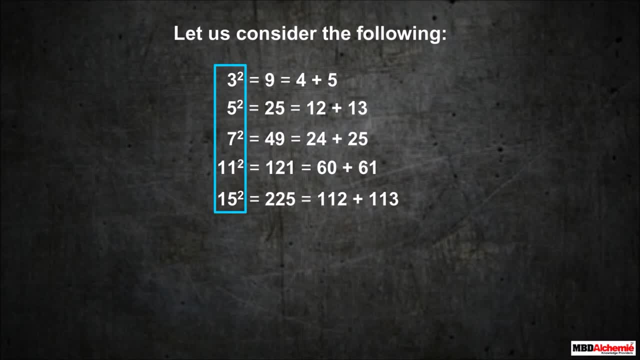 Let us consider the following. Let us consider the following: 1- the square of odd numbers as the sum of two consecutive numbers. We find the consecutive numbers by subtracting 1 and dividing by 2.. And we find another number by adding 1 and dividing by 2.. 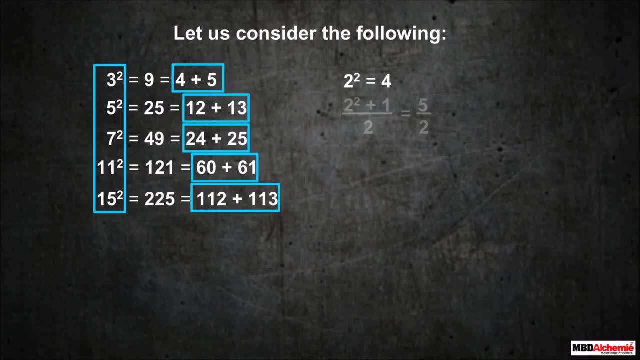 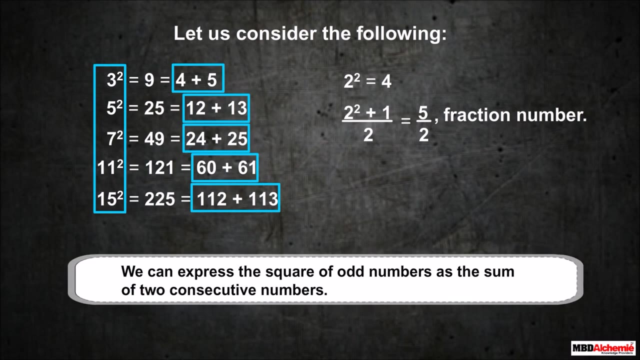 Now let's take the square of an even number. We find a fraction number instead of a natural number. So we say that this pattern is made only for square of odd numbers. We can express the square of odd numbers as the sum of two consecutive. 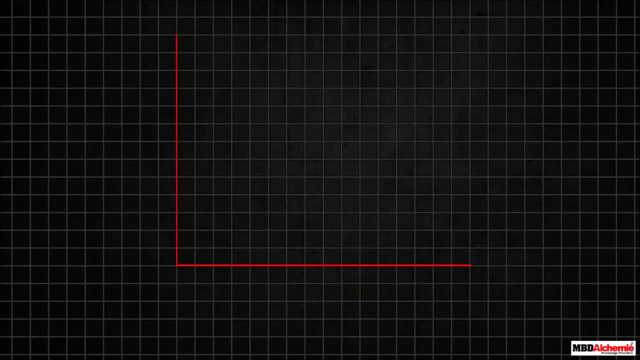 numbers. Let's see another property of squares. Consider a rectangle ABCD of length 30.. It has a length of 13 units and a breadth of 11 units. Now transform this rectangle into a square by cutting a rectangle of 1 unit breadth along the 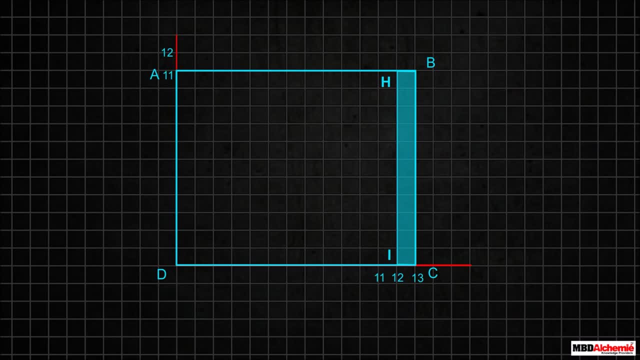 breadth BC of the rectangle ABCD, such that we get a rectangle HBCI. Now move and fix it along the length AH of the rectangle AHID. Observe the figure formed. Is it a square? How can this figure be made a complete square? 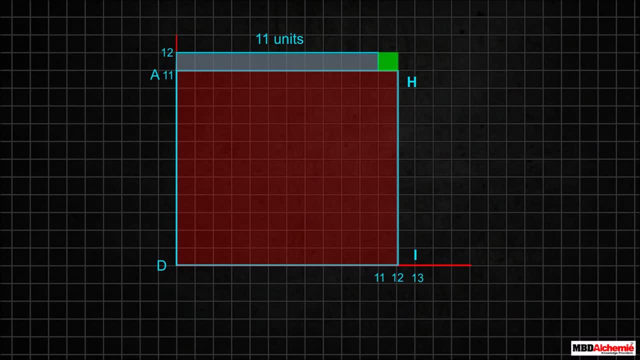 No, it's not a complete square, as there is something missing. Measure this missing space. This space can be filled by another square of 1 unit, As the rectangle fixed along the length is 11 units long, whereas the length of the shape left is 12 units. 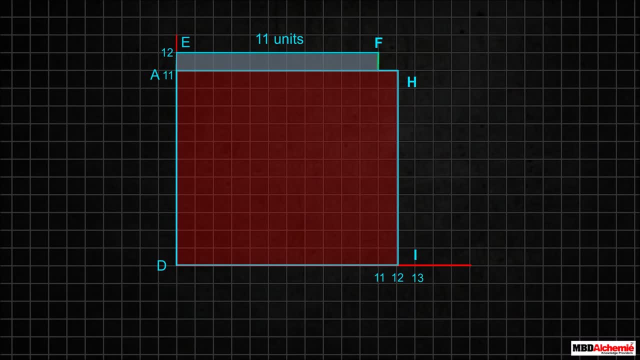 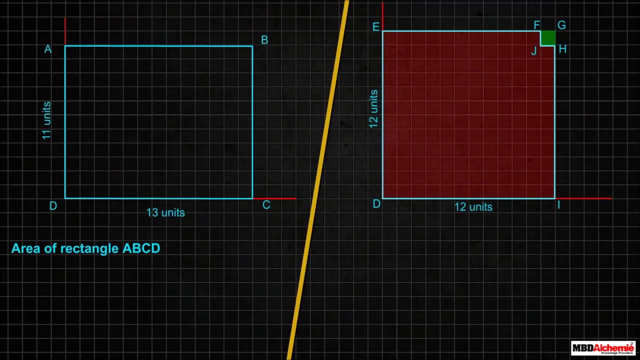 and the breadth of the rectangular cutout is also 1 unit. We know area of rectangle ABCD is length into breadth, ie 11 into 13.. This is equal to the area of square E, gloves of square EGID, minus area of square FGHJ, ie 12 square minus 1 square. Here we subtract the area of unit square from this square. this is equal to area of square EGID minus area of square FGHJ. Here we subtract the area of unit square from this square. this is equal to area of square EGID minus area of square EGID. Samsung Marine gauge. square area per minute square value. square to root of square means we have 12 square minus 1 square and we subtract the area of an even unit square, which is 12 to 12, will give us 12 unit square. Samsung Marine- good 수 zцен, do you agree? No problem, Simplify this. use conditions. 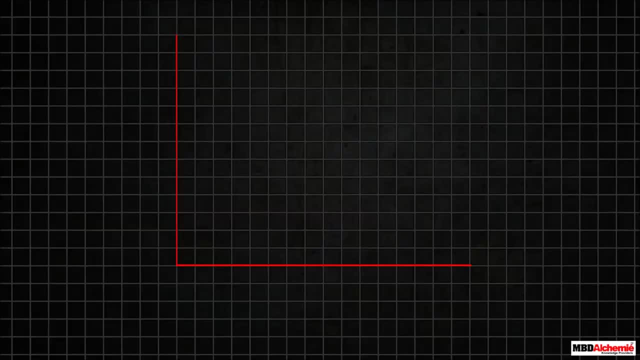 Let's see another property of squares. Consider a rectangle ABCD of length 13 units and breadth of 11 units. Now transform this rectangle into a square by cutting a rectangle of 1 unit breadth along the breadth BC of the rectangle ABCD. 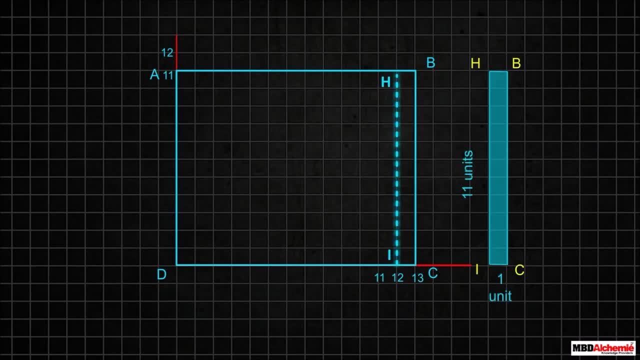 Such that we get a rectangle ABCD of length 13 units, Such that we get a rectangle HBCI. Now move and fix it along the length AH of the rectangle AHID. Observe the figure formed. Is it a square? 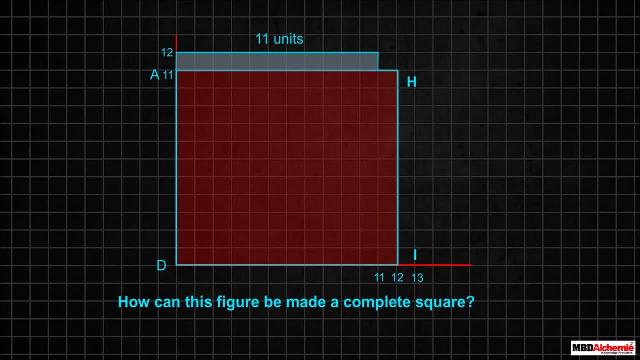 How can this figure be made a complete square? No, it's not a complete square, as there is something missing. Measure, Measure this missing space. This space can be filled by another square of 1 unit, As the rectangle fixed along the length is 11 units long. 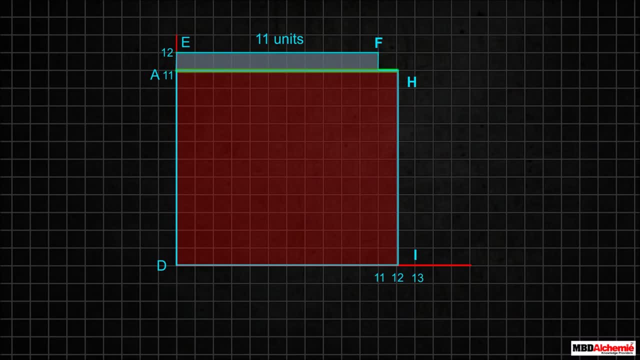 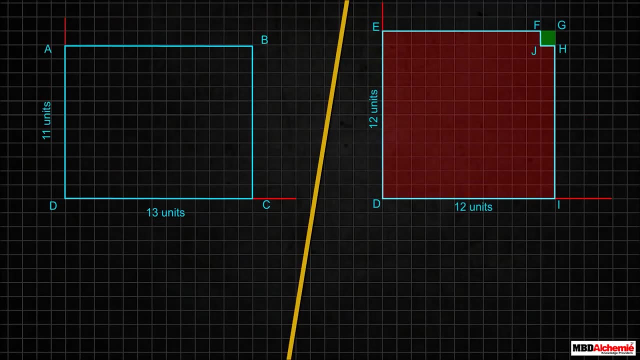 whereas the length of the shape left is 12 units and the breadth of the rectangular cut out is also 1 unit. We know area of rectangle ABCD is length into breadth, ie 11 x 13.. Now measure 12 x 1.. 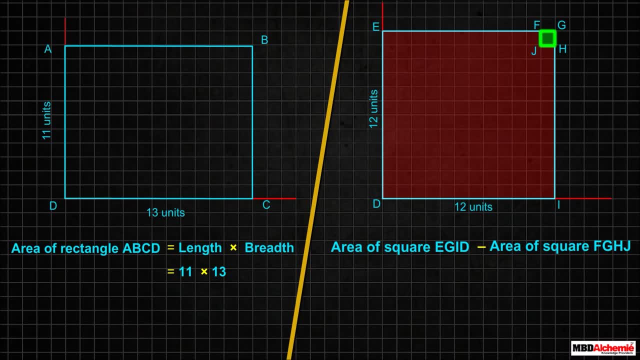 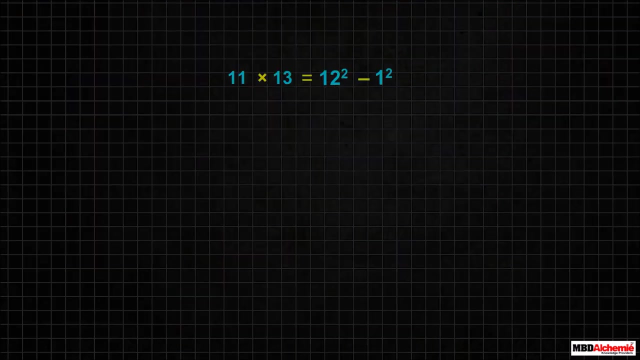 So 2 units square is equal to area of square HBC here, or 12x e with distance N, this square as 근 x1, trans Thema n s View 2.分 10 giving s 2, So two 1s plus 2s. 정 M H 2. The area of square HBCI is equal to EG i D absorbs area of square FG H J, That is 12 square minus 1 square. Here we subtract the area of unit square from the 12 square group, 12 square as the area of square formed as an additional unit square than the area of the original rectangle. 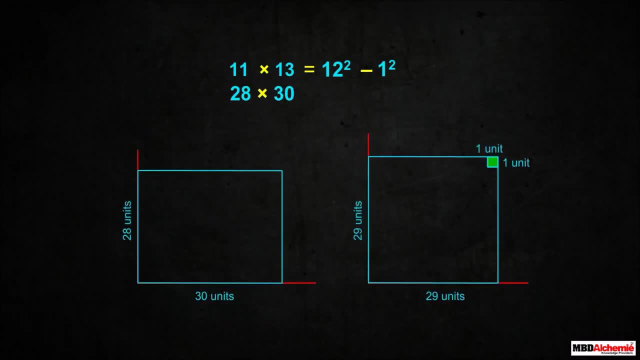 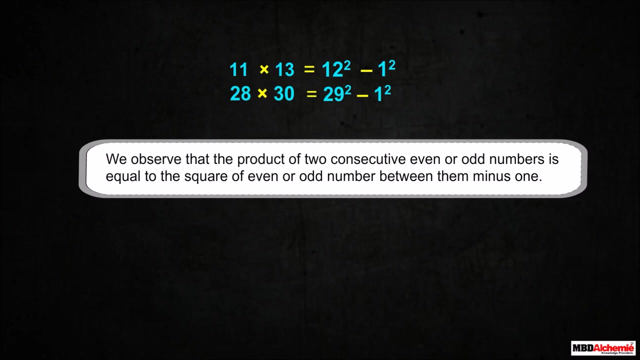 Similarly, the area of rectangle of sides- 28 units and 30 units- is written as the area of square of length 29 minus area of square of 1 unit. Do you observe any pattern here? Yes, we observe that the product of two consecutive even or odd numbers is equal to the square. 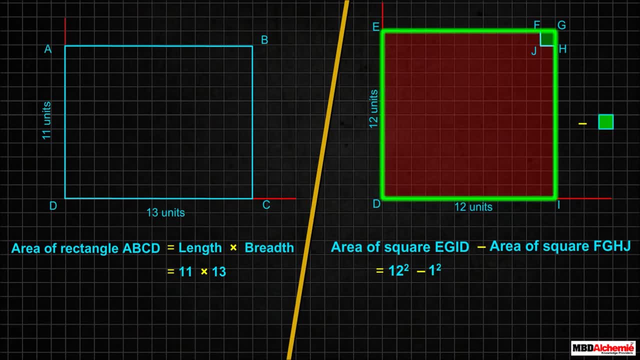 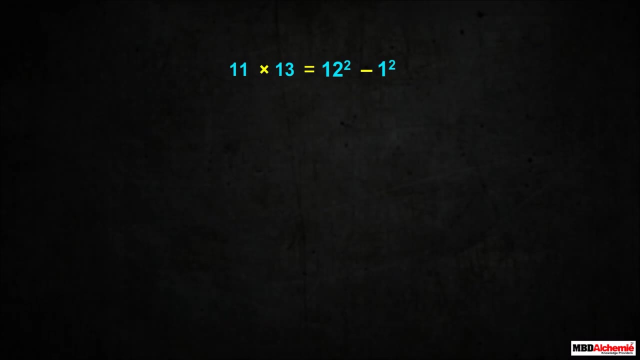 Read the diagram and collect information for chocolatelingue4.com. subtract the area of unit square from the 12th square, as the area of square formed has an additional unit square than the area of the original rectangle. Similarly, the area of rectangle of sides- 28 units and 30 units- is written as the area. 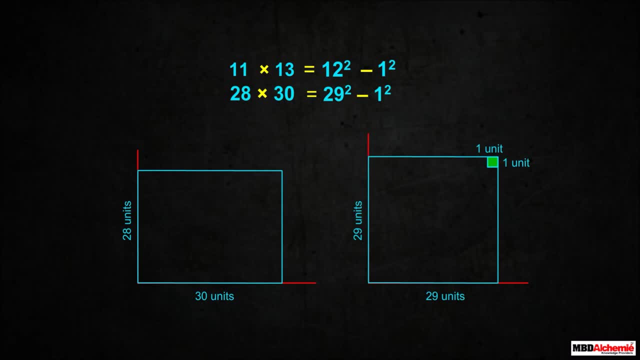 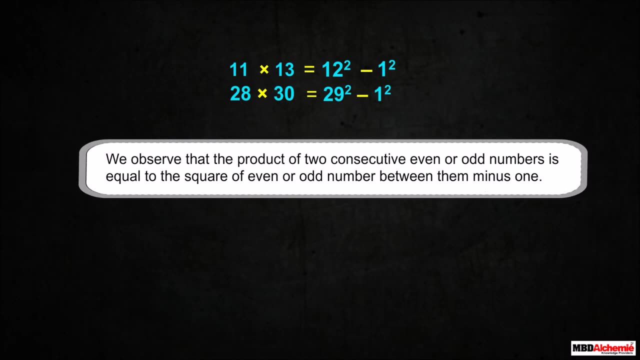 of square of length 29 minus area of square of 1 unit. Do you observe any pattern here? Yes, we observe that the product of two consecutive even or odd numbers is equal to the square of even or odd numbers between them, minus 1.. 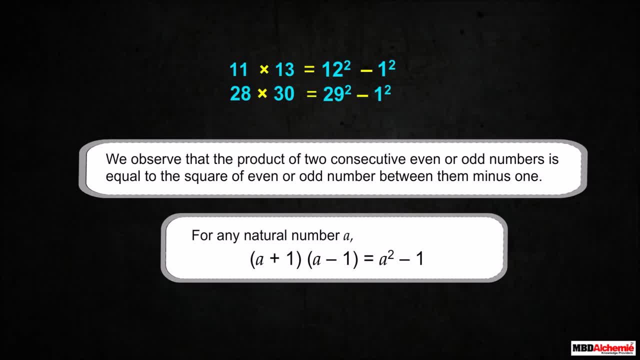 So in general we say that if A is any natural number, then A plus 1 into A plus 1 is equal to A plus 1.. So in general we say that if A is any natural number, then A plus 1 into A plus 1 is equal. 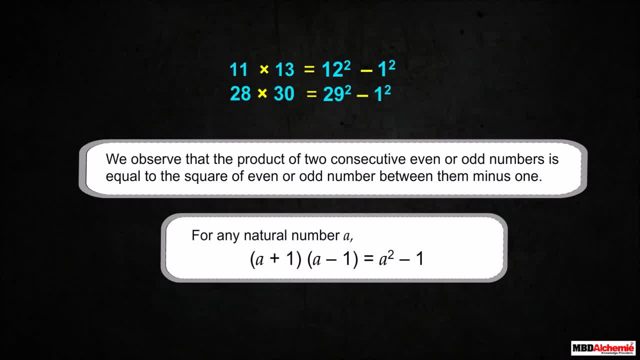 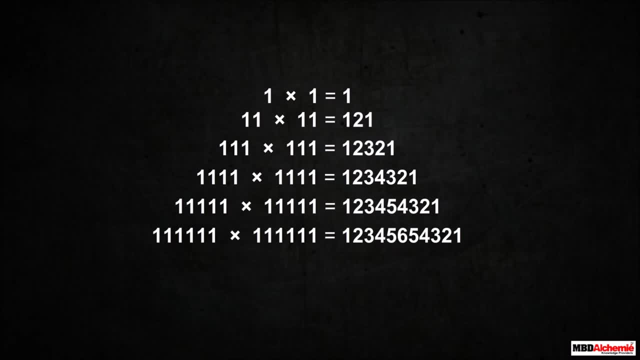 to A minus 1 is equal to A square minus 1.. Do you observe any pattern in this? First of all, the number of digits in the product is odd in number. Since the digit is odd, if we pick the middle digit, each side will contain even number. 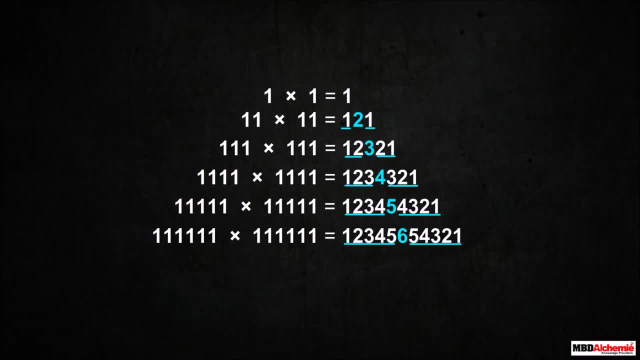 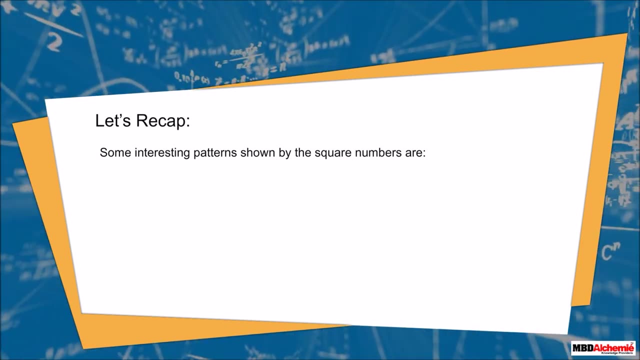 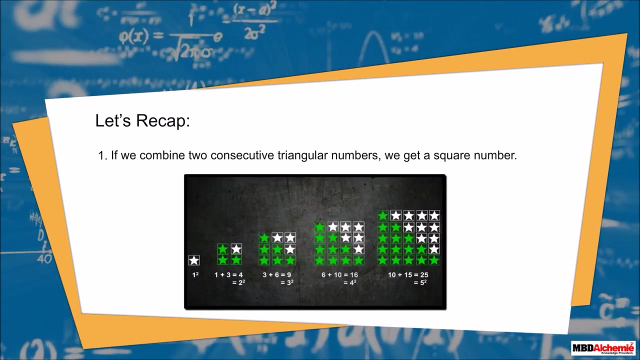 of digits and those numbers are in reversed symmetry. So all these are some patterns shown by the square numbers. Let's recap. Some interesting patterns shown by the square numbers are: If we combine two consecutive triangular numbers, we get a square number. 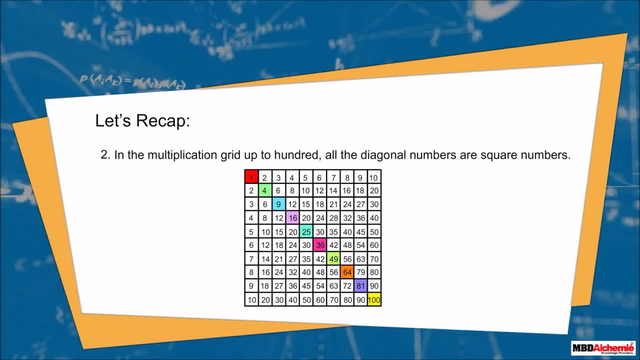 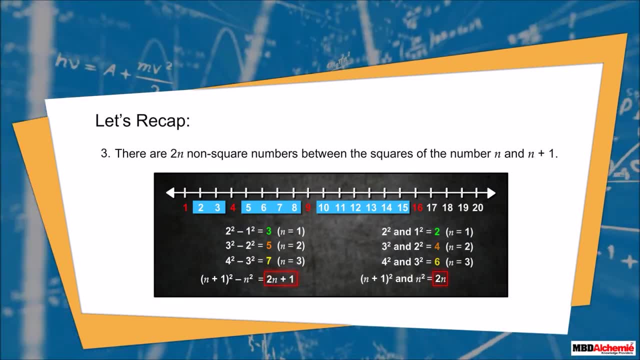 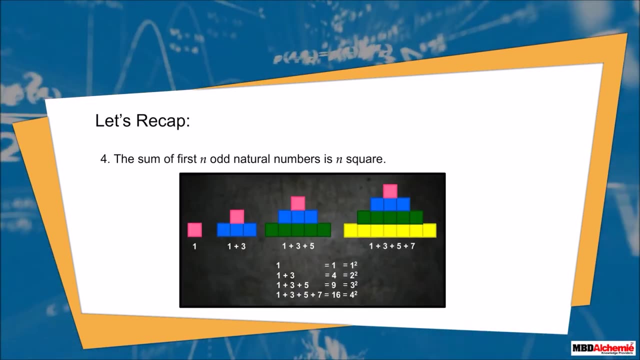 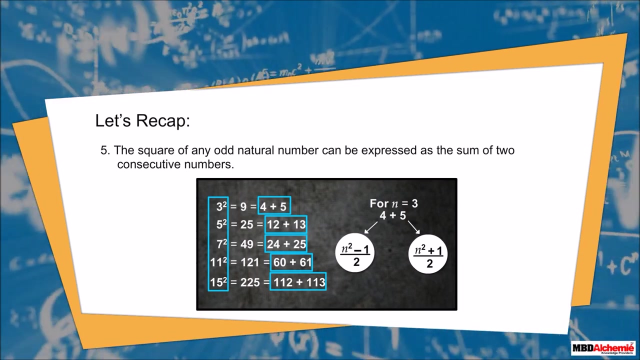 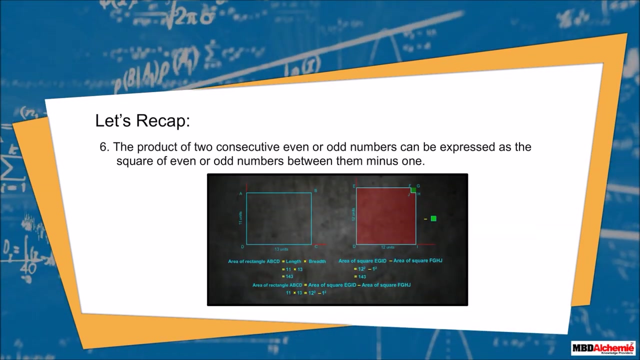 In the multiplication grid up to 100, all the diagonal numbers are equal to 1.. If we combine two quadrilateral numbers, we get a square number. If we multiply, the squares can beрp equal to 0.. Hence the same pattern.